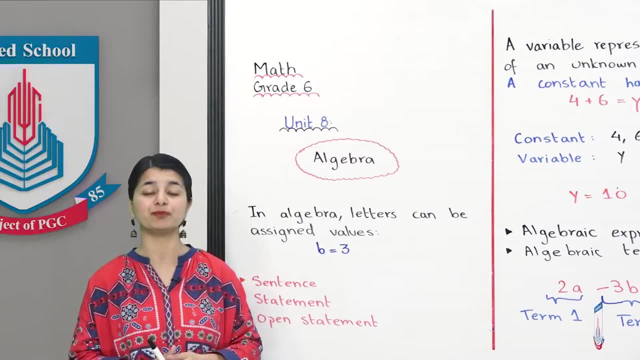 kyunki uske indar saari information aapko nahin di gayi hoti To kya divisions hai Sabse pehle there is a sentence in which aapko meaning convey kiya jaa raha hai kisi bhi? 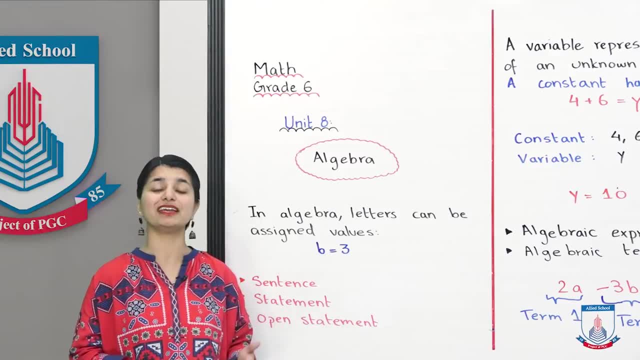 cheez ka. Phir statement: jo yaake true ho sakta hai, ya phir false ho sakta hai, and then we have an open statement, jisme aap determine nahin kar sakte, ki statement jo hai wo true hai ya false hai, kyunki aapke paas information missing hai. Ye main cheeze hamne shuru mein. 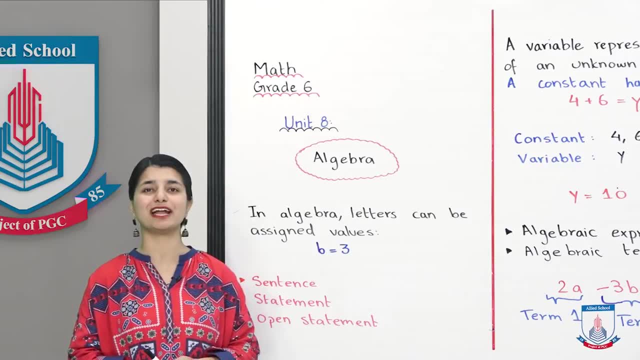 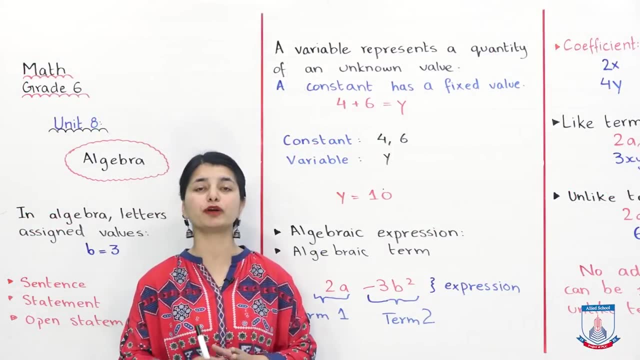 baat kerni thi, jink baare mein aage chalke aur terms ko seekte hai algebra se related. Ab algebra mein jo main cheeze aati hai, unme kuch terms hai, aapka variable, aapka constant. 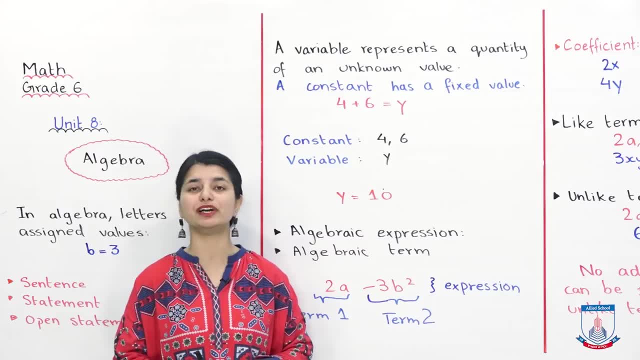 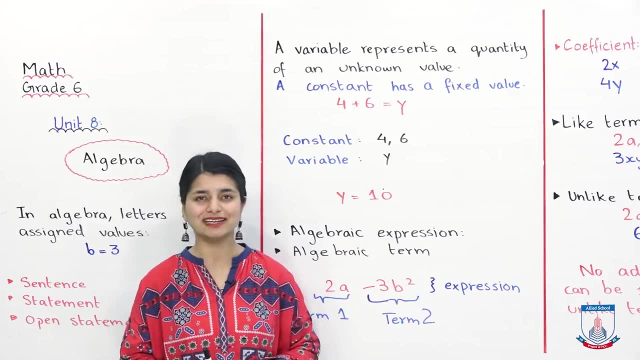 aapka coefficient. so these are some things that we will be learning about now. Sabse pehle ham dekhte hai, ki variable kya hota hai. Jab hamne baat kiya, ki ham letters ko value assign kar rahe hai, toh un letters ko basically ham variable kyahte hai. Vary karne, kya matlab. 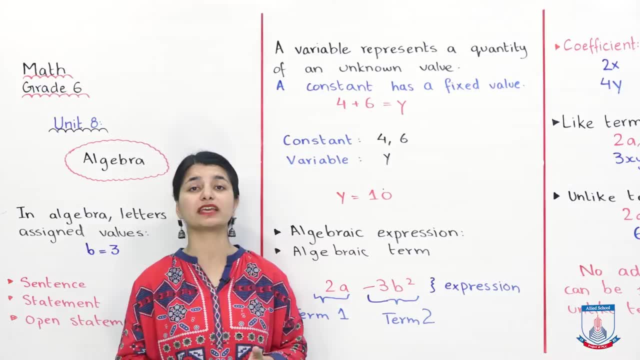 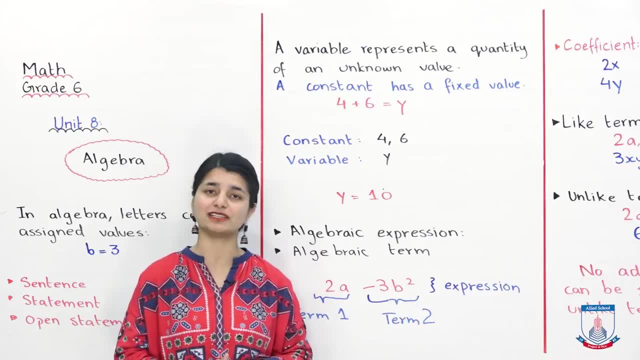 ka matlab hai eisi cheeze, jo change kar sakte hai, varie kr skte hai over time. Toh, jo letter aap likhte hai uskyi value, kuch bhi hot skte hai of apne, determine karni hai uskii fixed. 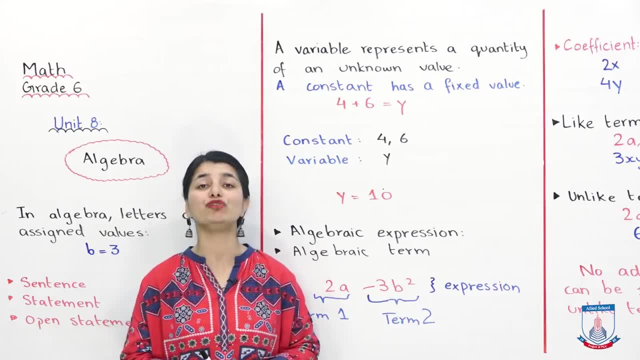 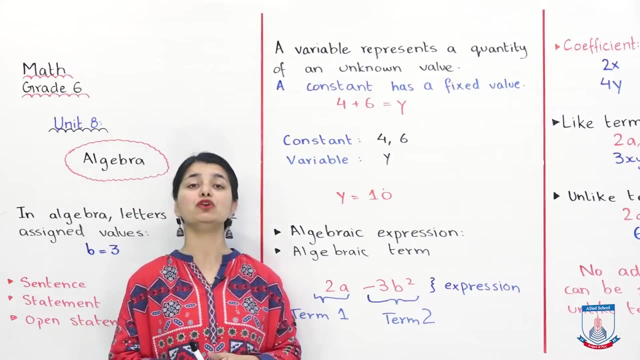 value aapko nahin di gai. Issli ham us letter ko variable kyahte hai. jası ki yaha par aap dekhiye a variant: represent a quantity of a unknown value. juss value ko aap nahin走吧. 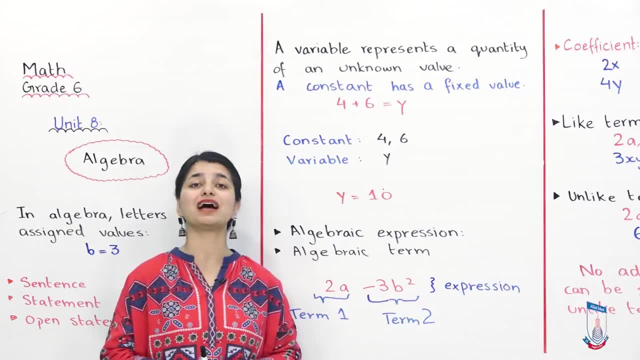 usko represent kerta hai variable aur ithme kuch bhi ahat skta hai, isme 12 ahat skta hai. it can have 12,, it can have 4000, and so on. Next, if we see what is constant. 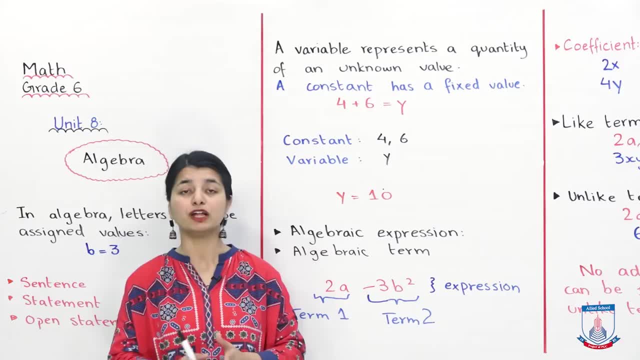 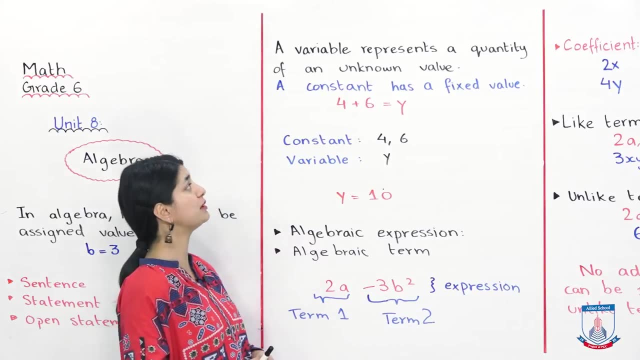 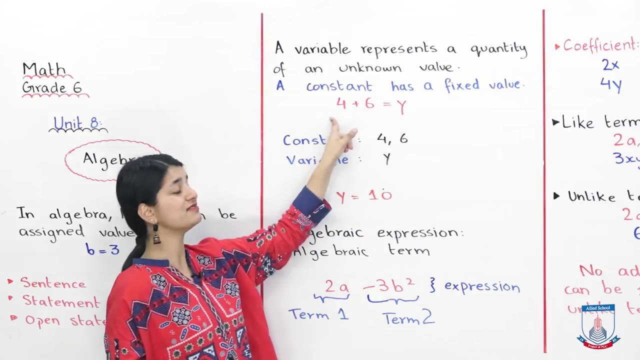 Constant is its fixed value. So when we write a statement, one thing is constant and the other thing is variable. For example, if we see this statement: 4 plus 6 equals Y. Which things have fixed value here? 4 has fixed value and 6 has fixed value. 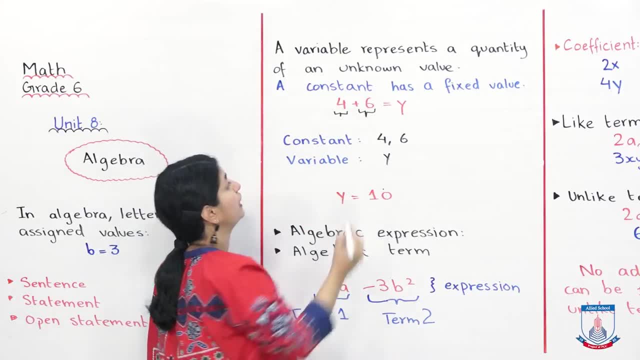 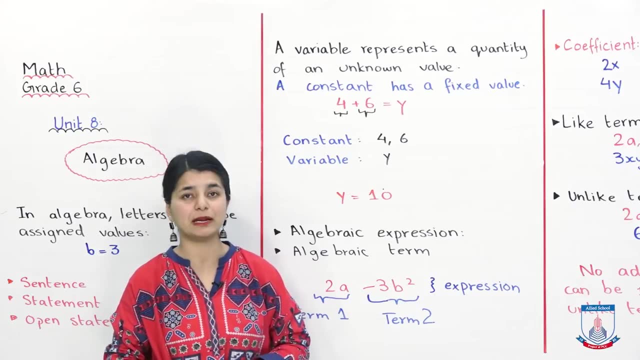 because you cannot change it. So these two have become our constant, Whereas Y can have any value, You have to find out its unknown value. So our constant is 4 and 6 and our variable is Y. Now the question would be: 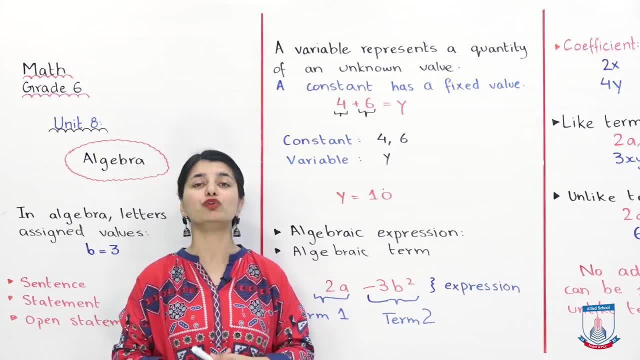 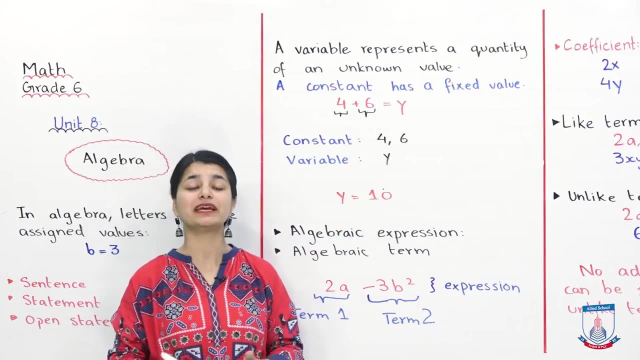 that you find out the unknown value of Y. So how will you do that? By solving it. So when you add 4 plus 6, you figure out its answer: 6 plus 4 is 10.. So Y's value is 10.. 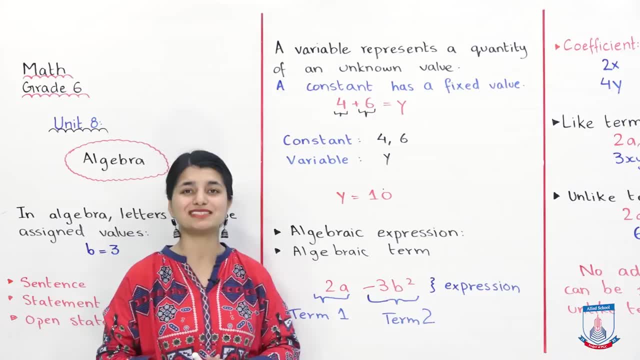 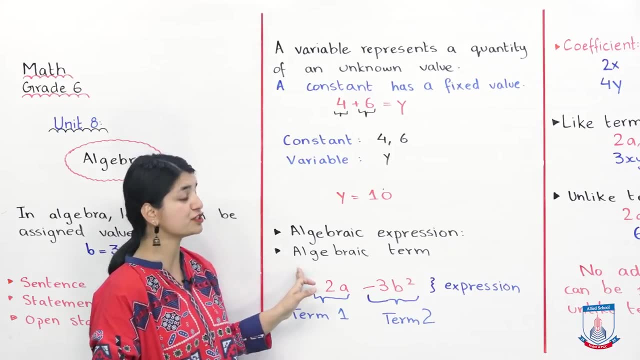 Interesting. In this way, we can solve our variables. We have some constants and some variables. This way, we can solve equations. Next, we are looking at what is an algebraic expression and what is an algebraic term When you use operations. 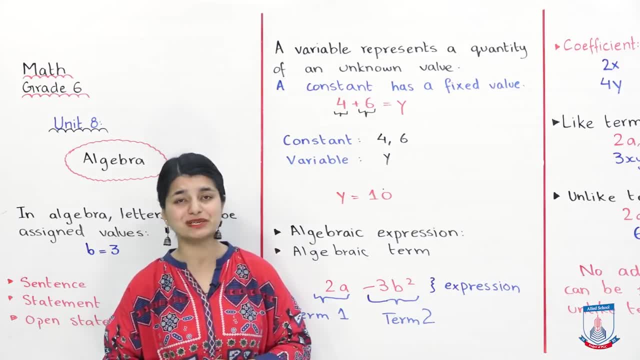 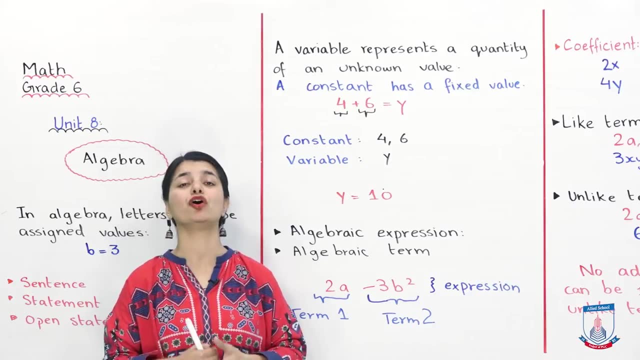 between the letters, variables and constants. with algebra, What are the operations? in maths There are 4 operations: Addition, subtraction, multiplication and division. So when you use these operations between the algebraic terms, it is called an algebraic expression. 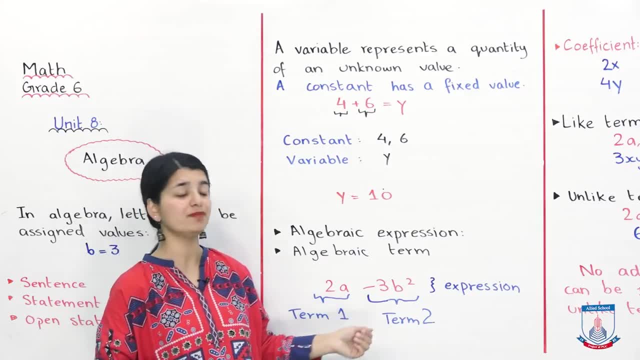 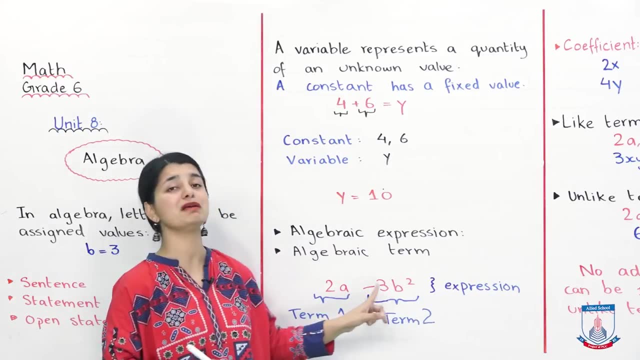 As you can see here, For example, you have this statement: 2a minus 3b square. To solve it or to express it in this term, because there is a minus in the middle, this will be called an algebraic expression. 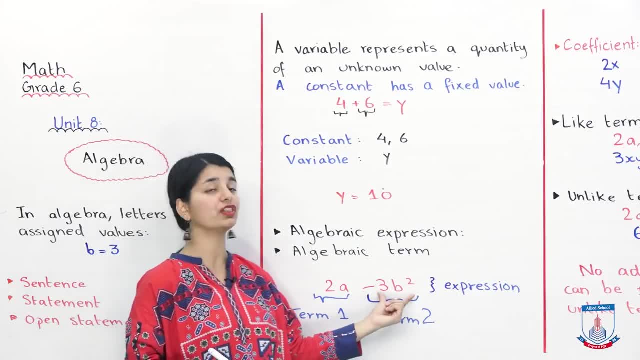 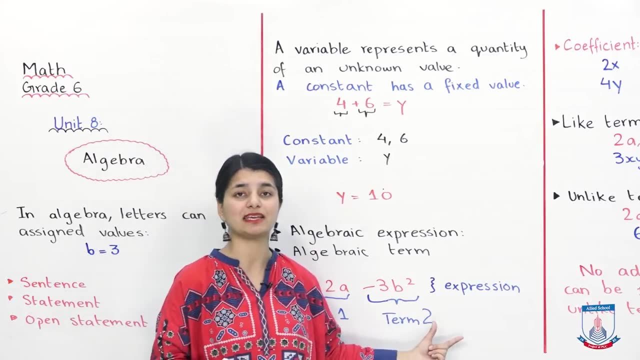 But if you see these two separately- 2a and 3b square, minus 3b square, because its sign will also come with it- these two will be called our algebraic terms. So the whole thing, the whole thing. 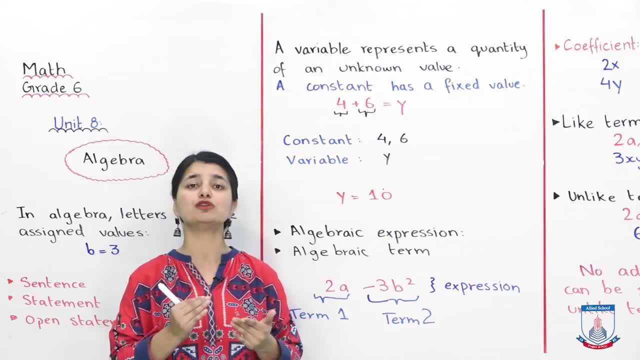 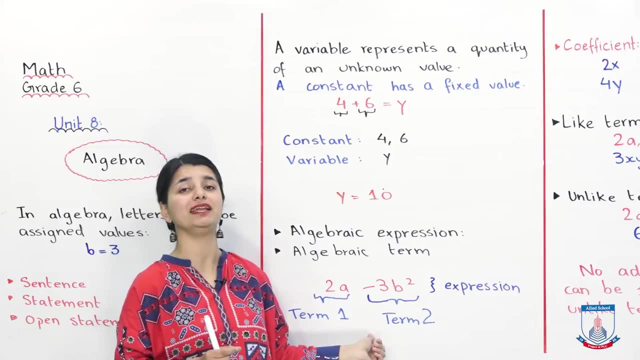 is a figure in which operations are used. We call it our algebraic expression And the terms made with different variables in it, we call them our algebraic terms. So over here we have one term that is 2a and another term that is minus 3b square. 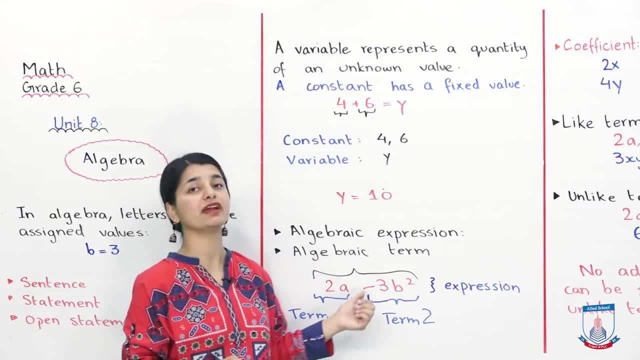 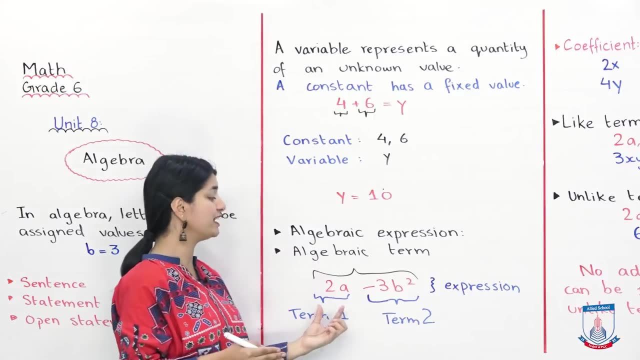 And by combining this whole thing, we call it our algebraic expression. This whole thing is ours because an operation is being used between it. This is our algebraic expression, Whereas these two different terms are our algebraic terms. So this is our algebraic expression. 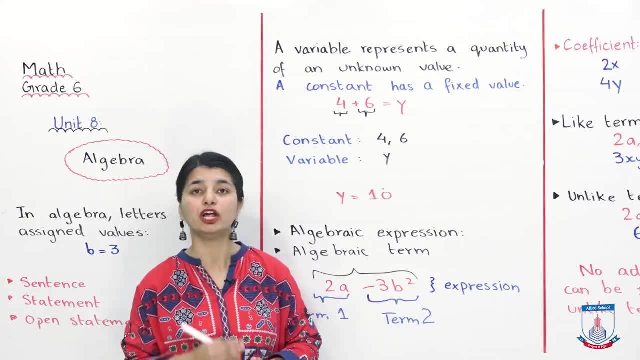 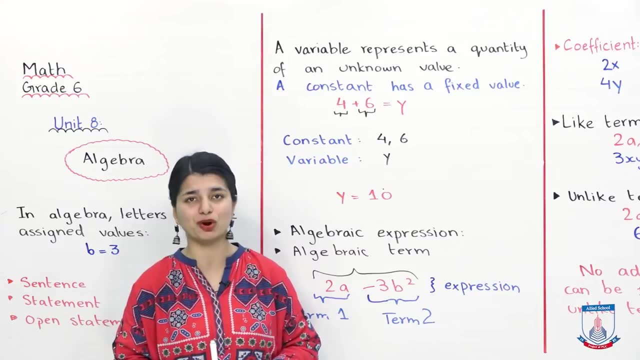 So this is our algebraic expression. If it was written here plus 4a, then it would be our third term. If it was written here plus 11y, then it would be our fourth term, and so on. Come, let's go ahead and understand some more terms. 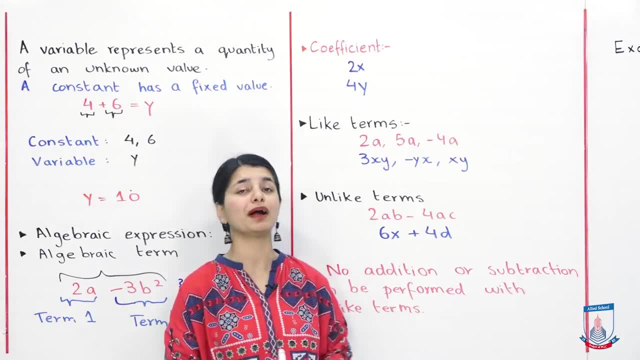 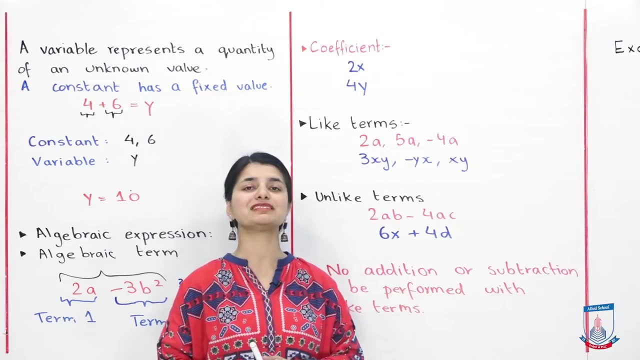 The next term that we have to talk about is coefficient. So what is our coefficient? Coefficient is the number that comes with your variable. The first example we did, it had constants. Concepts are completely different, Like 6 plus 4 equals to y. 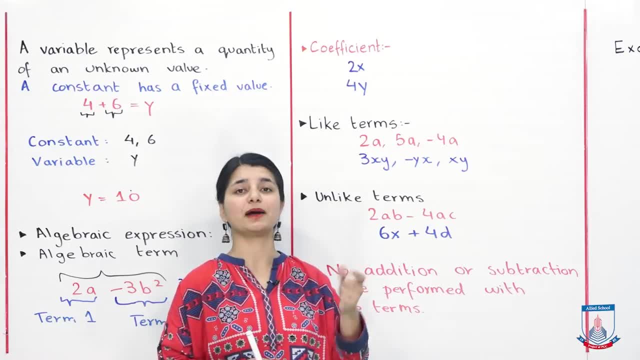 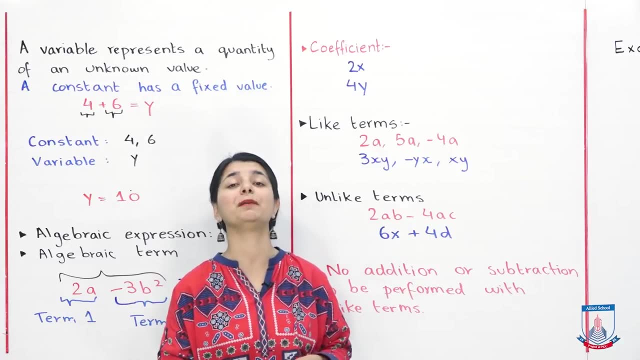 So 6 is a constant because it is alone. 4 is a constant. If it was written there 350, then it would be a constant. But when a number comes with a variable, then it is our coefficient Before the variable. 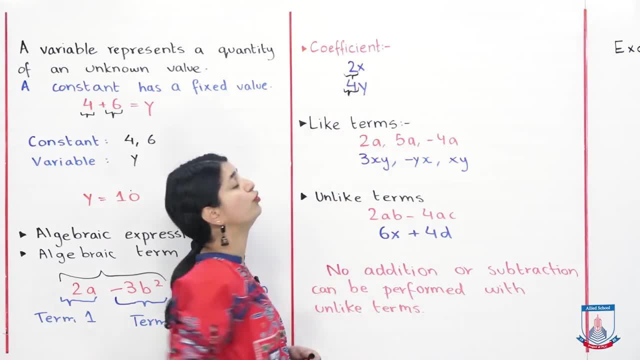 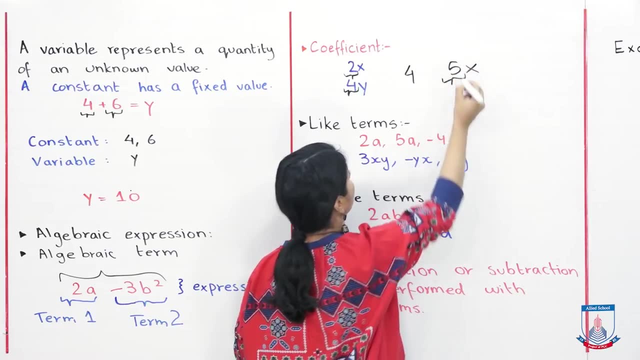 So 2 is our coefficient, 4 is also our coefficient. This would be a constant, but 5x in this, 5 would be our coefficient. 5x in this 5 would be our coefficient. 5x in this, 5 would be our coefficient. 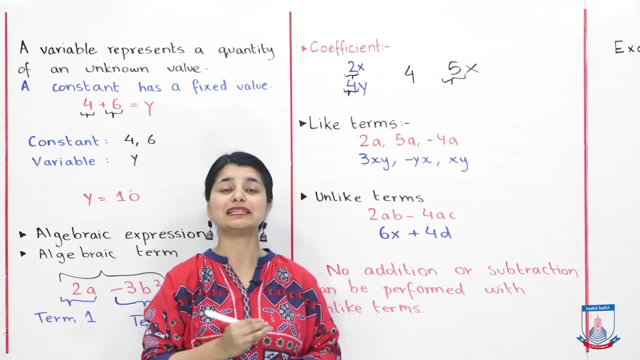 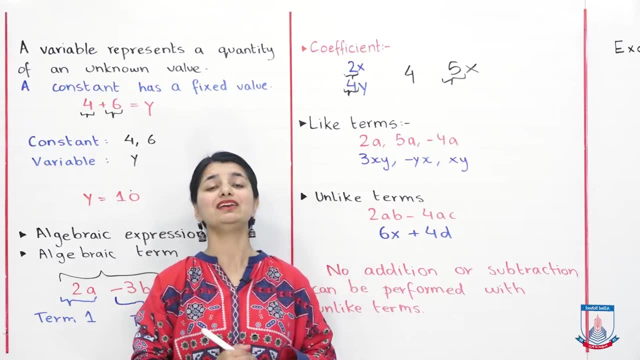 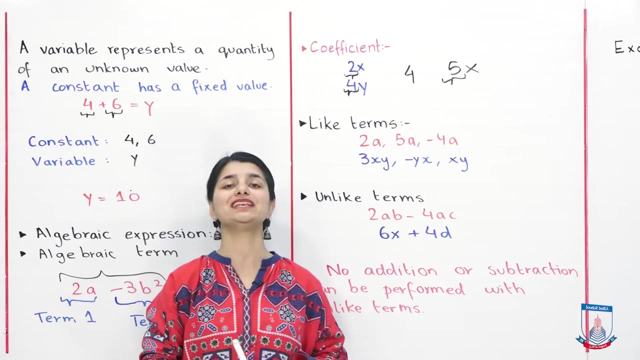 In this way, whenever there's a number before a variable, that is called our constant Looking ahead. we have to talk about like terms and unlike terms. Like terms are those where your variables remain the same even though the numerical values don't vary. 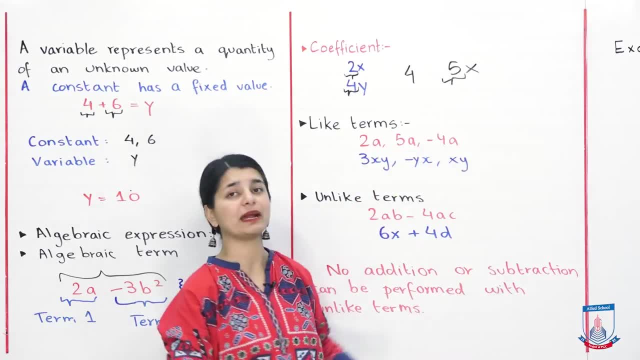 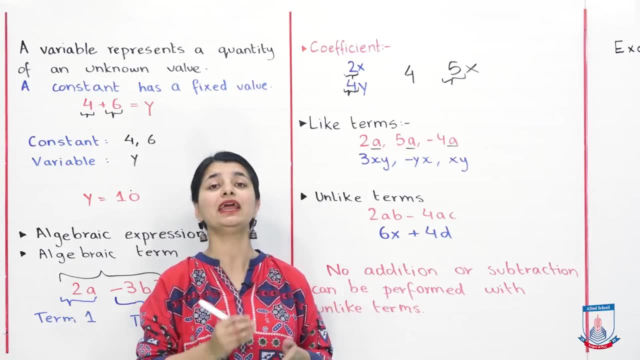 For example, 2a, 5a and minus 4a. all of them have a. So all the terms between all of them become like us. So all the terms between us become like us. you can add these, subtract these, you can interrelate these, you can interact with them. 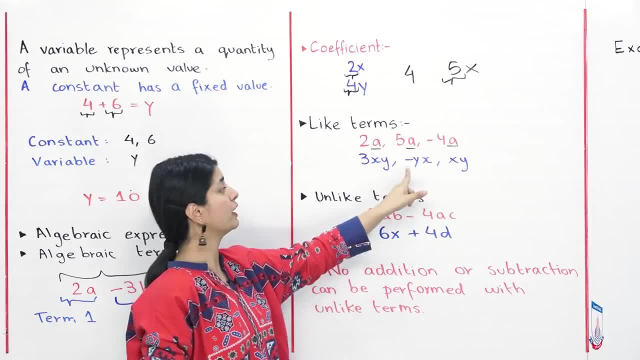 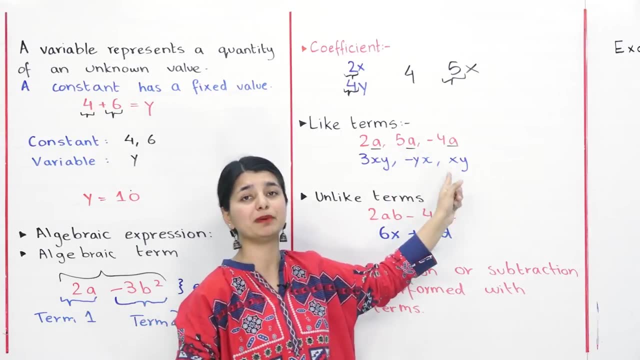 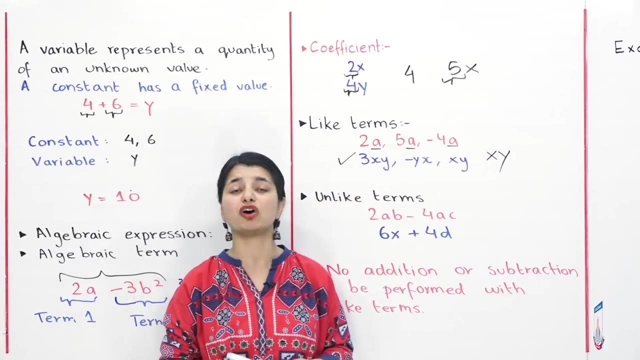 second option is 3xy minus yx, xy. of course y is written first and then x, but because all three have the same variables, xy, common in all three, xy, so these are called like terms and you can solve these: add these, subtract these. 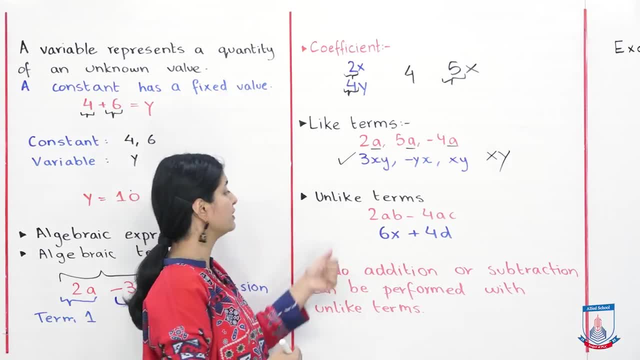 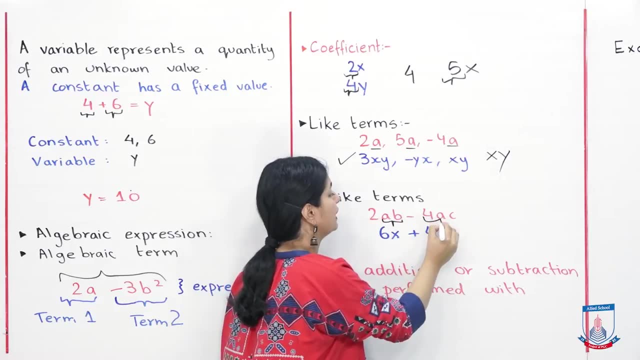 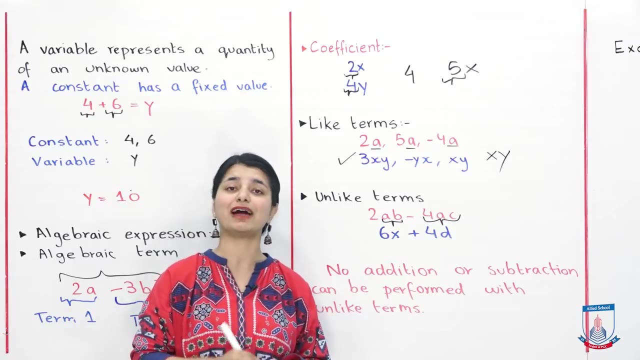 unlike terms are opposite to this, as you can see: 2ab minus 4ac. in one place ab is there, in other place ac is there. so these are unlike terms. they cannot be added, subtracted, multiplied or divided further. 6x 4d. 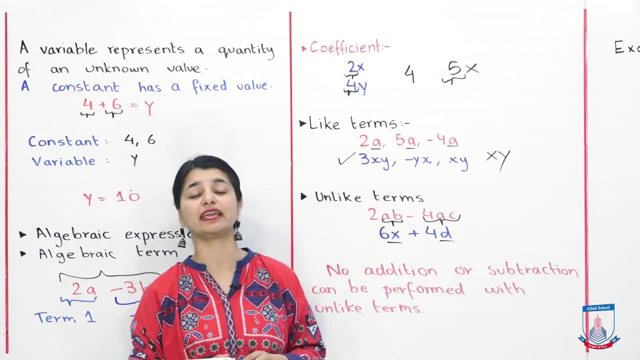 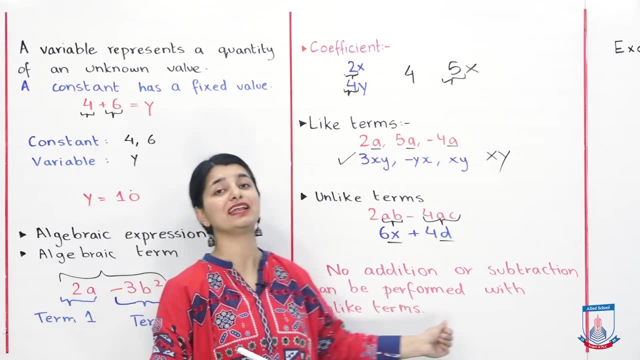 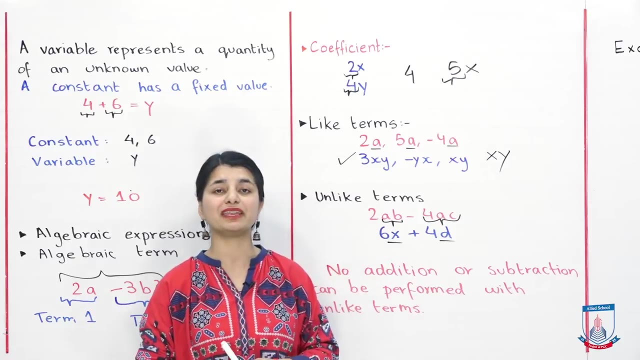 so x and d are unlike terms and they cannot be added or subtracted from one another. no addition or subtraction can be performed with unlike terms. so what happens? you cannot do addition or subtraction with unlike terms. what we will do now is we will do their examples. 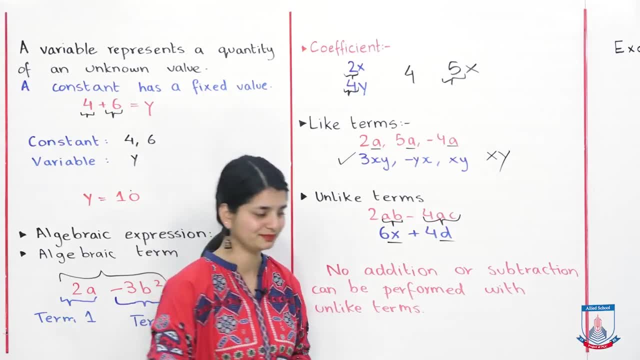 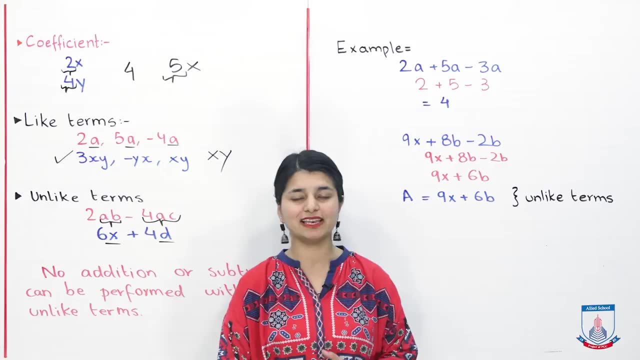 so that you can understand the difference between like and unlike terms. let's see the basic examples so that you can prepare for your exercise 8a. so the first example is 2a plus 5a minus 3a. a is coming in all three. 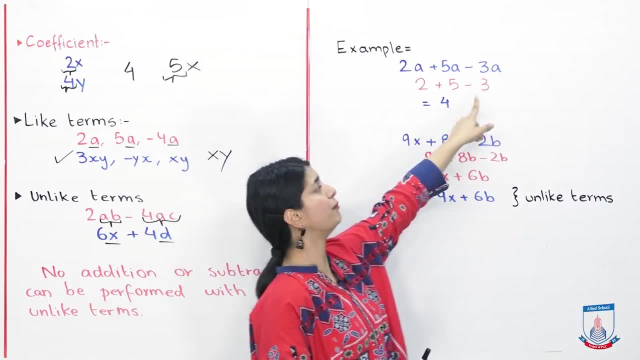 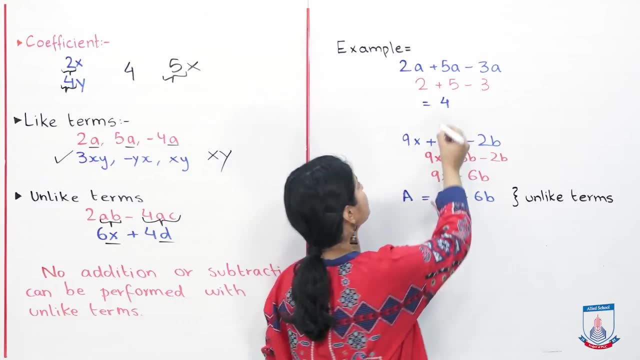 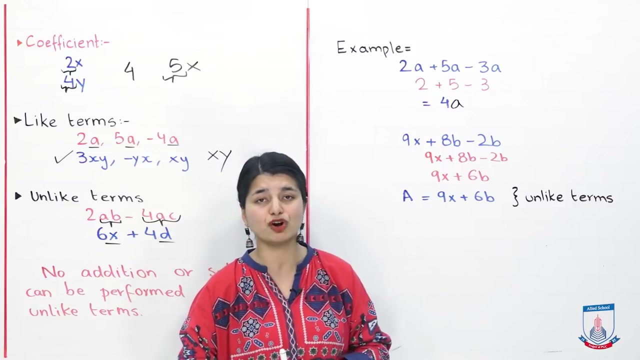 which means all three are like terms. so 2 plus 5 minus 3, simply you have to do. you can ignore a. your answer is 4 and once you have your answer you can add the variable which was common in all. these were like terms, so we easily solved this algebraic expression. 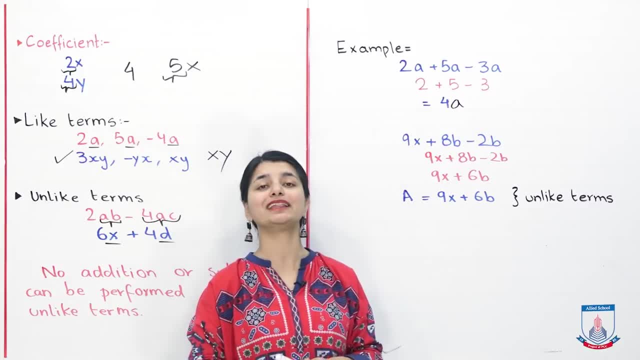 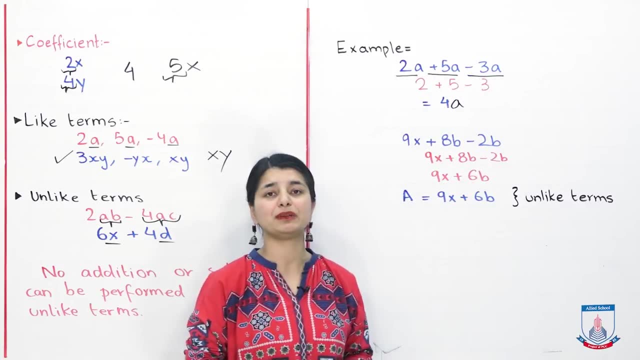 this whole thing was our algebraic expression, and how many terms are there in it? there are three algebraic terms: 1,, 2 and 3. in this way, we have identified our algebraic expression and our algebraic term in the second example you have. 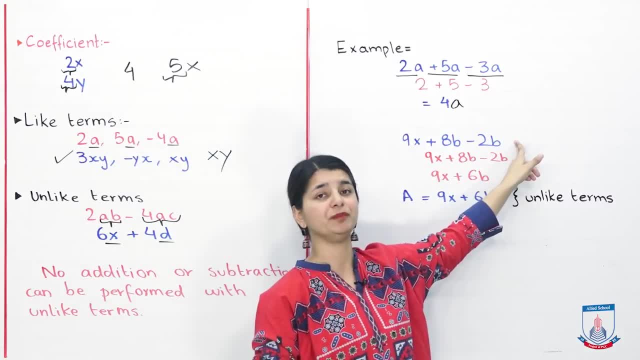 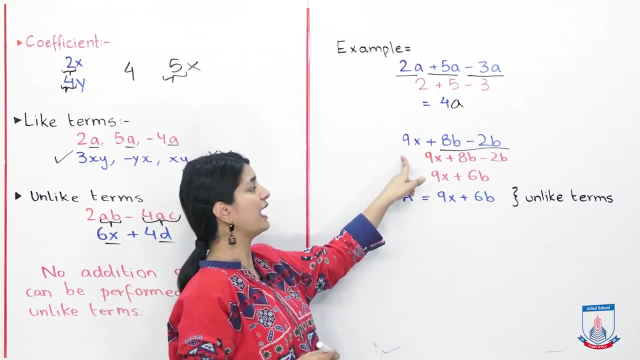 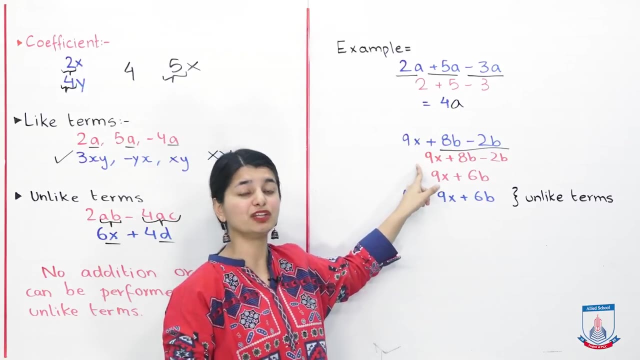 9x plus 8b minus 2b. now here, two terms are like terms. these two terms are like terms, right, but the term with x is not like them. so if you start solving them, 9x will remain the same, because no addition or subtraction can be performed with unlike terms. 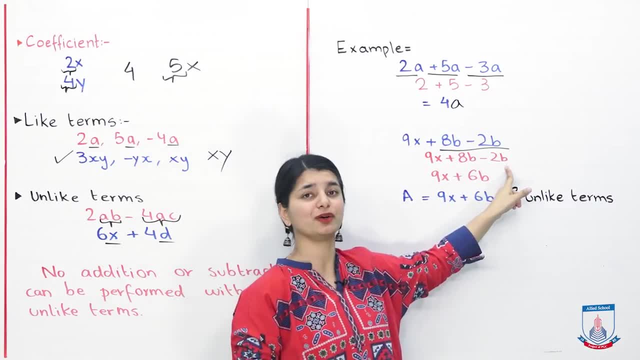 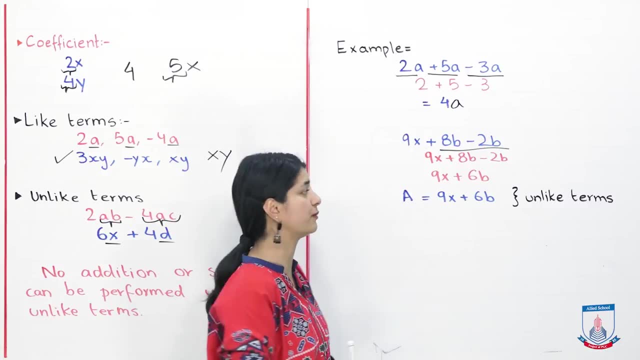 so you can do minus 2b from 8b and that will result in plus 6b, but you change 9x with this. you cannot add or subtract with this, so you have two terms left and your final answer would be 9x plus 6b. 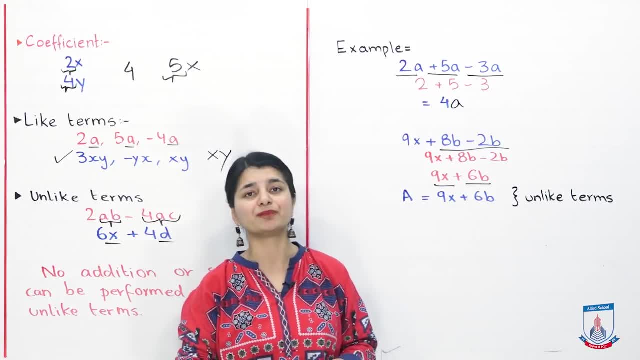 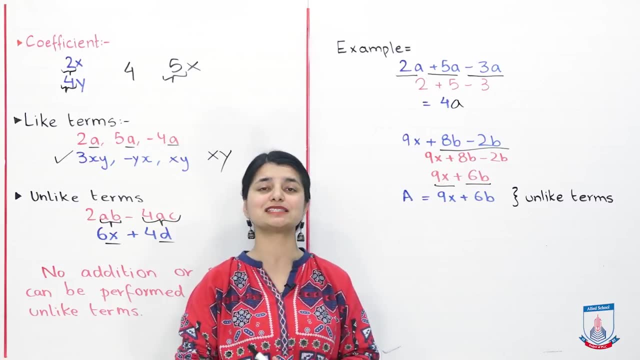 which is an algebraic expression, and you cannot solve this further. with this our lecture ends today. we just had to do introduction with algebra so that you get acquainted with all the terms. now we know what is sentence, what is statement, what is open statement, what is variable.